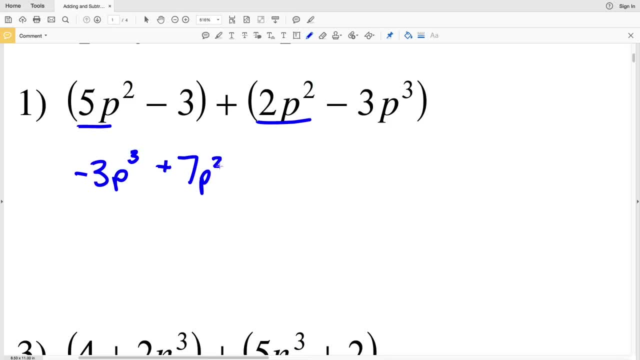 So that's 5 plus 2, which is 7p squared, And then finally subtracting that, 3.. So negative 3p cubed plus 7p squared minus 3 is the answer and number one. A rule of thumb when writing a polynomial is to write it with the greatest exponent towards the left. 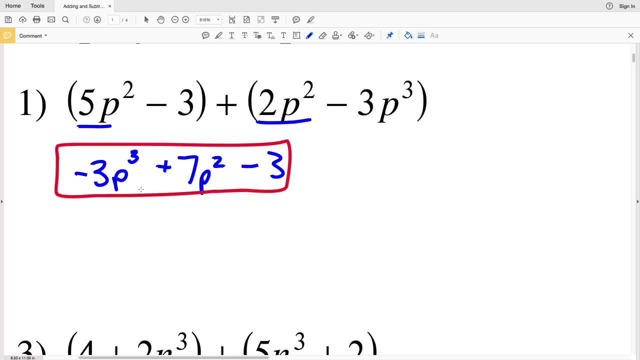 and then going in descending order as you go to the right. So we have our p cubed, then our p squared, Then if we had a single p we would put that in, and then the constant. Let's move on to number two. 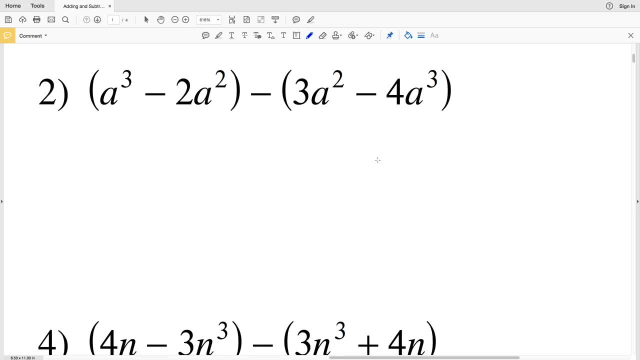 Now we know that addition is commutative, meaning that the order that we add terms in doesn't matter. However, subtracting the 3a squared minus 4a cubed is the same as adding a negative 3a squared minus 4a cubed. 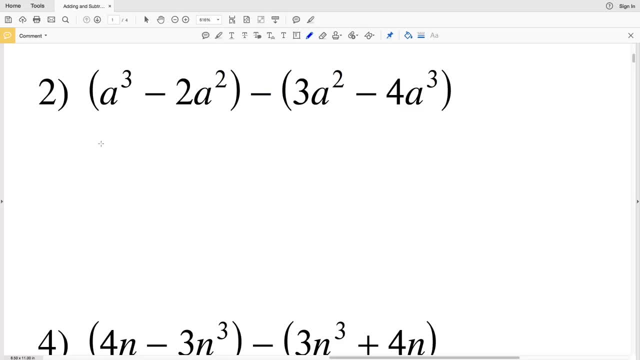 And if we're adding a negative of that, that means that this can be rewritten as a cubed plus negative 2a squared, plus distributing that negative negative 3a squared, plus distributing that negative again, a 4a cubed. 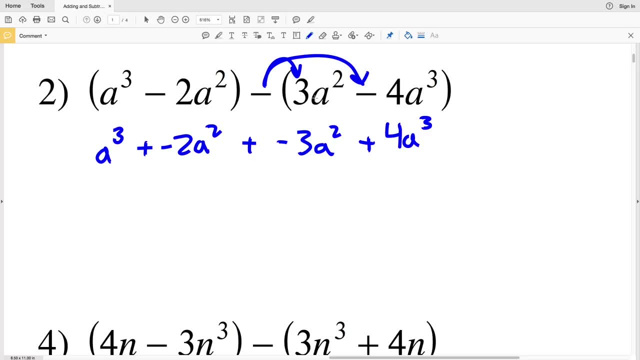 So since this term is negative, or we're subtracting that positive, the 3a squared becomes negative and the 4a cubed becomes positive. Now let's go ahead and combine our like terms. We can combine the a cubed with the 4a cubed. 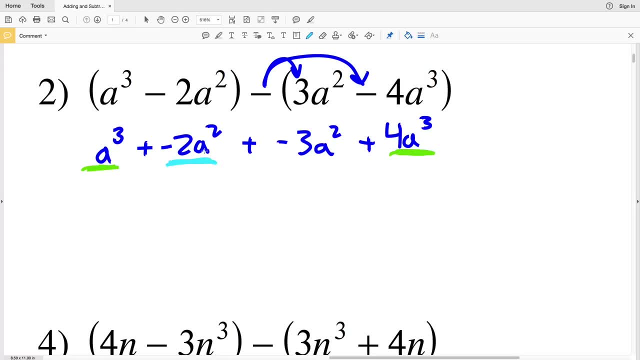 and we can also combine the negative 2a squared with the negative 3a squared, since the exponents are similar. a cubed plus 4a cubed is like 1a cubed plus 4a cubed, which will give us 5a cubed. 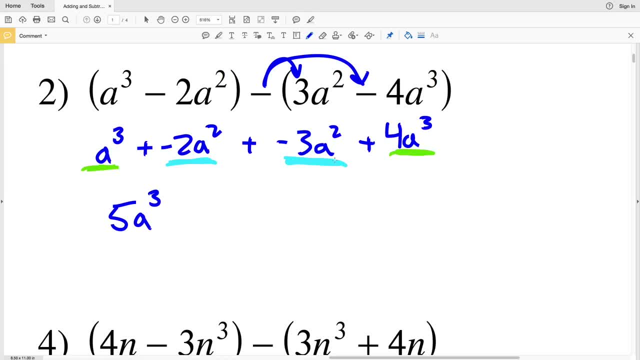 And then negative 2a squared plus negative 3a squared equals negative 5a squared And since we have a 4a cubed, we can combine that we're adding a negative. that's the same as subtracting a positive. so the answer for number 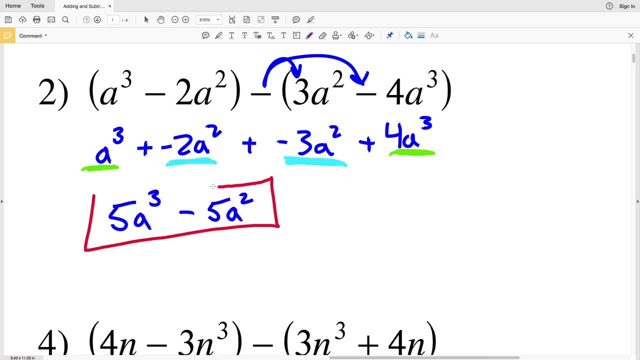 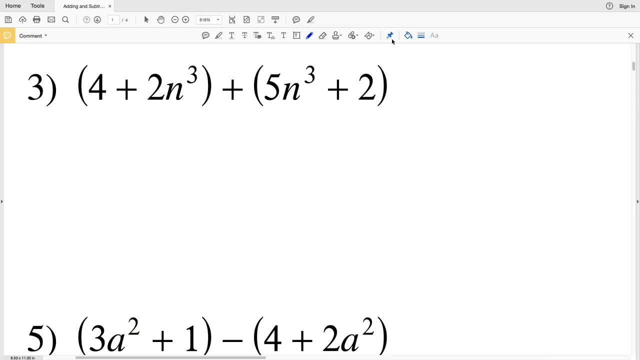 two is five a cubed minus five a squared, and number three: it's all addition, so we don't have to worry about distributing. a negative are similar terms. we have two constants of four and a two and we have two in cubes. we have two times into the three and five times into the three, so combining: 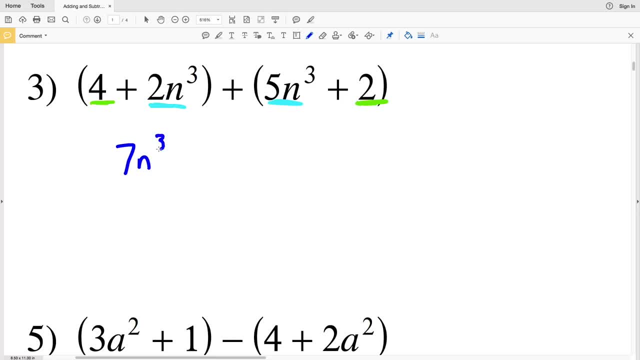 those first, we'll get seven n cubed plus four plus two is six. seven n cubed plus six is the answer in number three. moving on to number four, we are subtracting terms and remember subtracting is the same as adding the negative. so I'm going to go ahead and distribute that negative right. 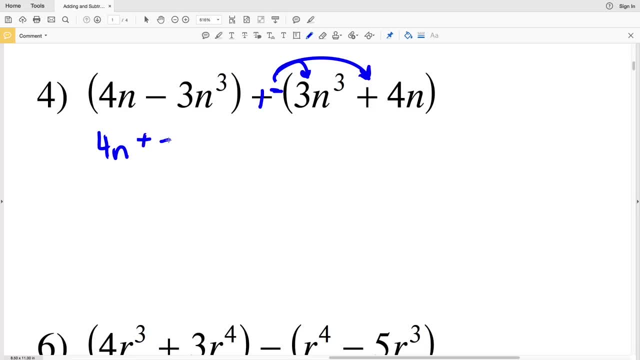 away. I'll rewrite this as four n plus a negative three n cubed plus a negative three n cubed again plus a negative four in. now combining like terms, I have a positive four n and a negative four n, and I also have a negative three n cubed and another negative three n cubed, combining the. 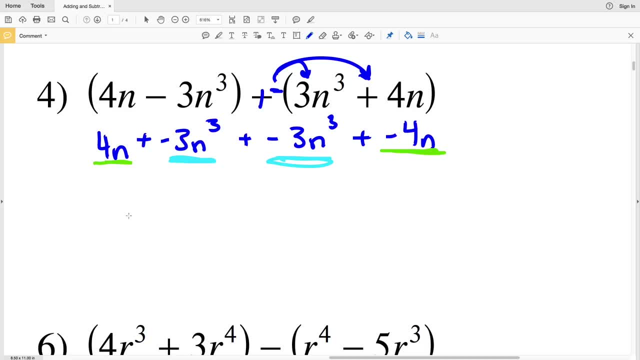 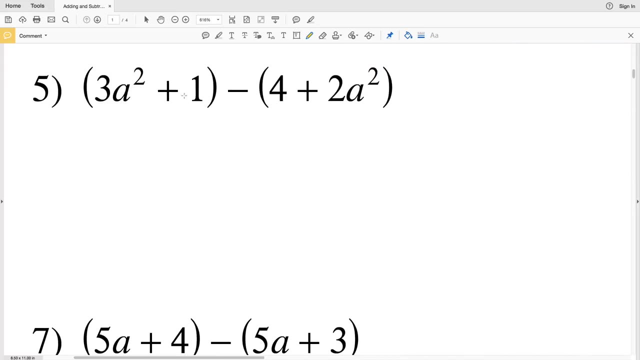 negative three n cubes. first negative three plus negative three is negative six. so I'll have negative six in to the third and then four n plus negative four n is zero. so my final answer for number four is negative six n cubed and number five, again, I'm going to add the negative and then 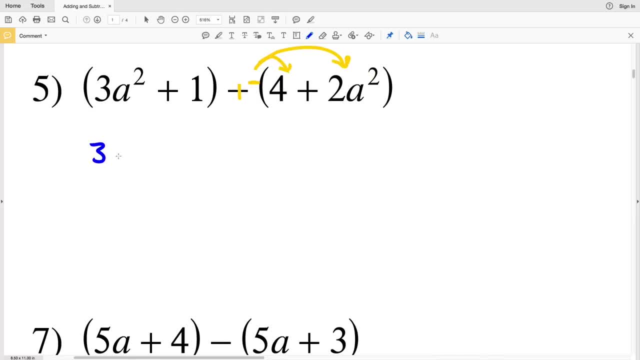 distribute that so it's going to be three a squared plus one plus negative four plus negative two a squared. and now you can see that, combining like terms, I have three a squared and a negative two a squared and I have two constants, one and negative four. combining those three a squared plus a negative two a squared will be a positive one a squared. 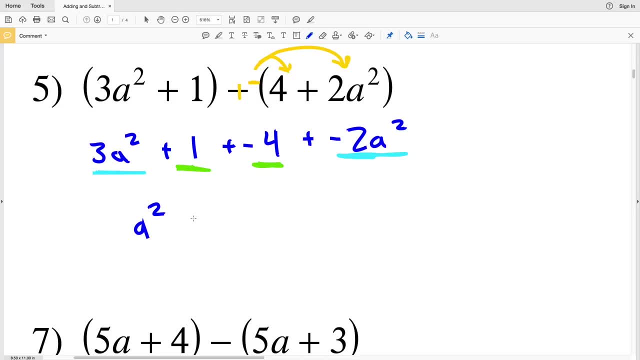 which is simply a squared, and then a positive one plus a negative. four will leave me with a negative three, and when you add a negative it's the same as subtracting that positive. so a squared minus three is the answer. in number five, number six: again, I want to distribute that negative one. 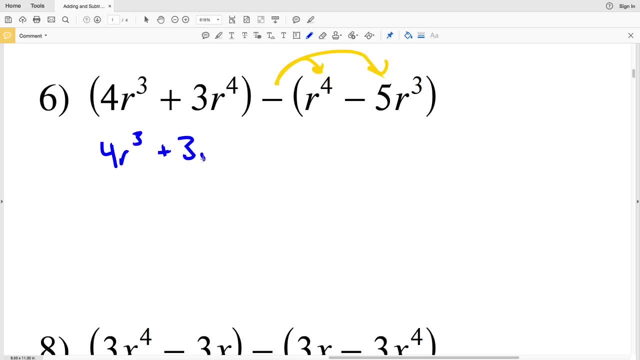 so I'm going to have four r cubed plus three r to the fourth, plus a negative r to the fourth plus a positive five R cubed, combining like terms. I have two terms with R cubed and I also have two terms with R to the fourth. an exponent of four is greater than three. 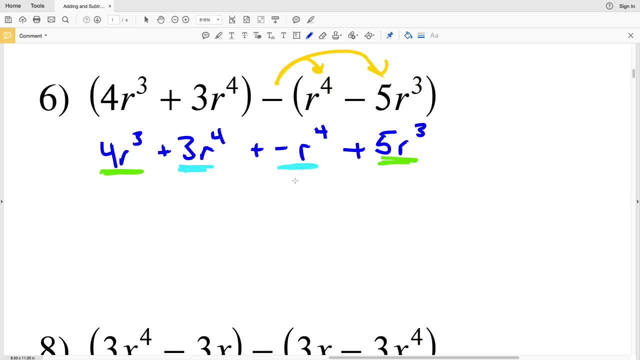 so I'm going to write that term first. three are to the fourth. minus R to the is 2 R to the fourth. and then we have 4 R cubed plus 5 R cubed, which is 9 R cubed, so 2 R to the. 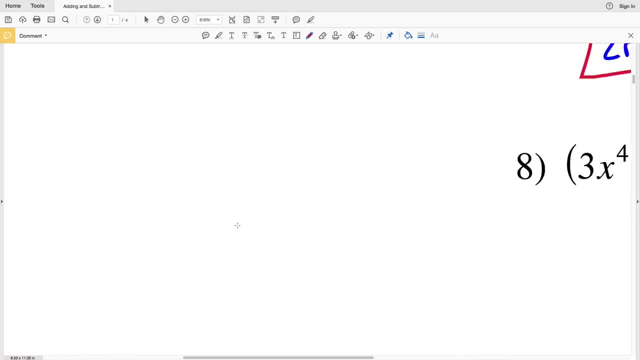 fourth plus 9 R to the third. moving on to number 7, again we're adding a negative, 5 a plus 3. so we're going to have to distribute that negative to the 5 a and to the 3, so we'll have 5 a plus. 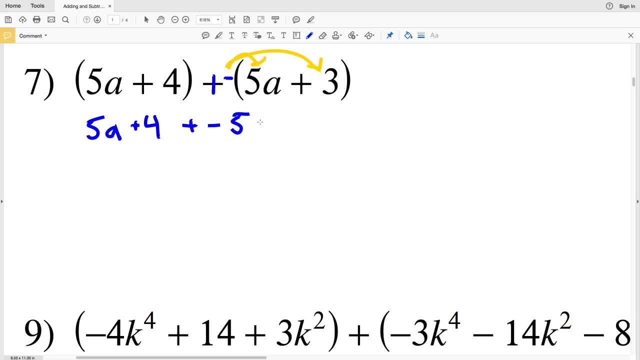 4 plus a negative 5 a plus a negative 3, combining like terms. we have to combine the 5 a together and we're going to have to combine the constant together. 5 a plus a negative 5 a is 5 a minus 5 a, which is 0. so these will cancel out and then we'll have 4 plus a negative 3, which is the same. 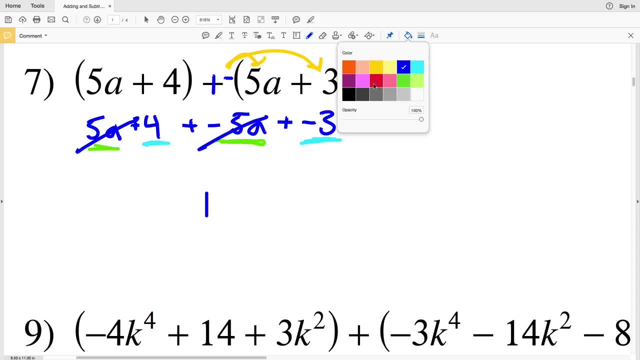 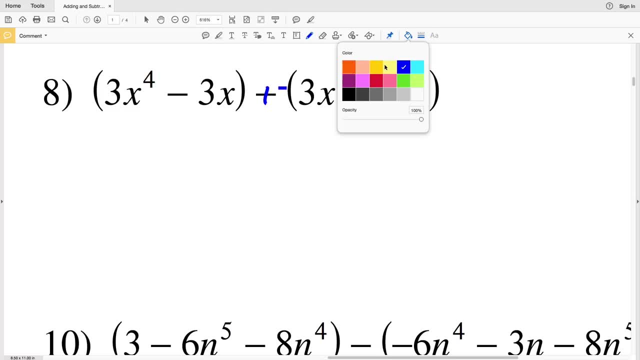 as 4 minus 3, which is a positive 1. so, simplifying this expression, we get a solution of 1 and number 8. again, I'm going to start by distributing that negative and you don't have to do that, but it makes it easier to remember. 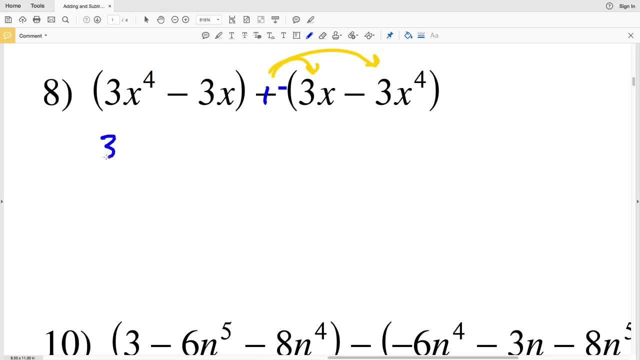 whether you're adding or subtracting those terms. so I'm going to say 3x to the fourth plus a negative, 3x plus a negative, 3x plus a positive, since the negative times the negative is positive to the fourth. now, combining like terms, I have 3x to the fourth and I have another 3x to the fourth. I 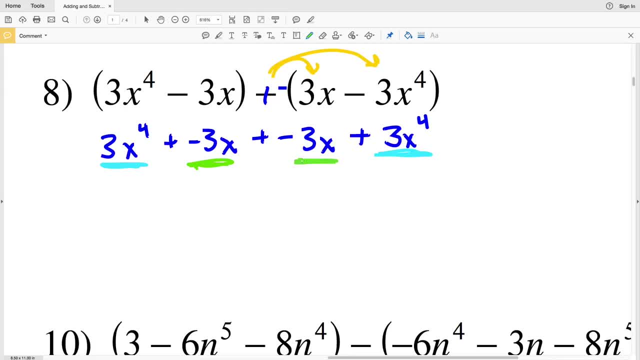 have negative 3x and a negative 3x. so I have two terms where the exponent is 4 and I have two terms where the exponent is 1. doing the exponent of 4 first, I'll do 3x to the fourth plus 3x to the. 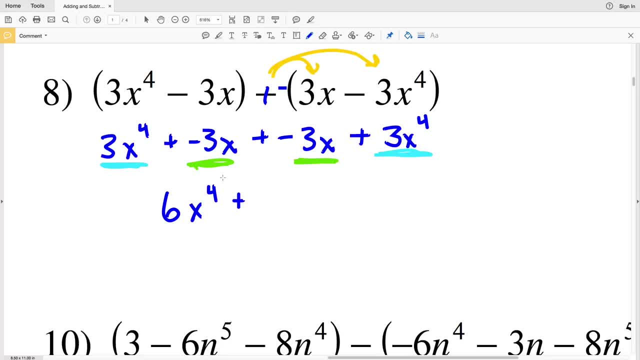 fourth, which is 6x to the fourth, and then I'm adding a negative 3x plus negative 3x, which is a negative 6x. but we know that when we're adding a negative it's the same as subtracting that positive. so 6x to the fourth, minus 6x for number 8 and number 9. for combining like terms. we're 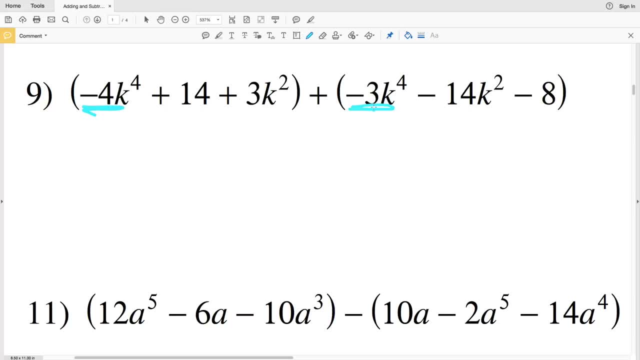 going to combine the negative 4 K to the fourth and the negative 3 K to the fourth. we're then going to combine the constant of 14 with the constant of 8, and we also are now going to combine this 3 K squared with the other K squared, starting with the greatest. 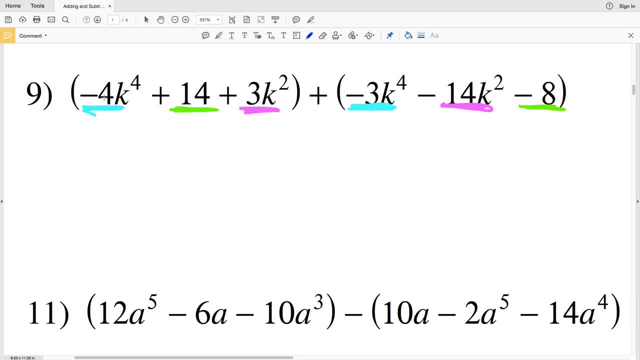 exponent value the 4, we're going to combine negative 4 K to the fourth and negative 3 K to the fourth to get negative 7 K to the fourth. since negative 4 plus negative 3 is negative 7, then we're going to combine the next greatest exponent, which is 2, so 3 K squared plus negative. 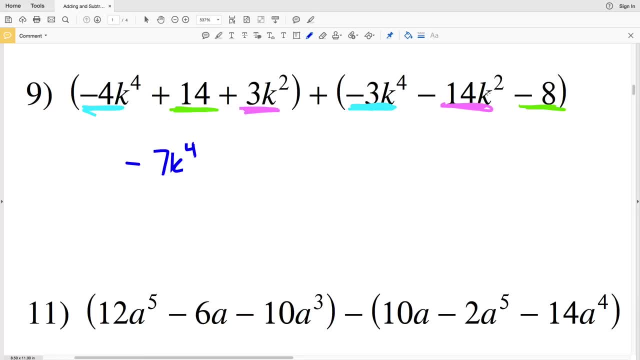 14 K squared is going to be subtracting 11 K squared, so negative 7 K to the fourth, minus 11 K squared, since 3 K squared plus negative 14 K squared is negative 11 K squared. and lastly, we're going to combine the constant 14 plus a negative 8 is going to give us a positive 6, so 14 minus 8. 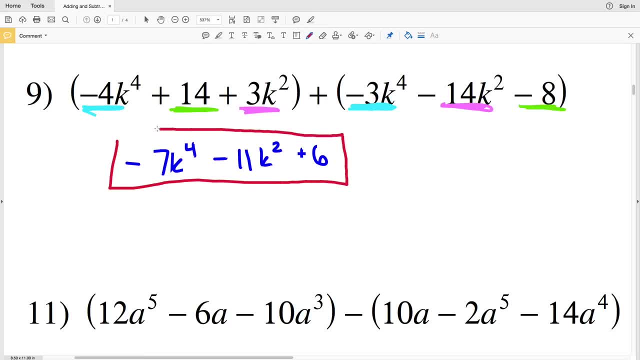 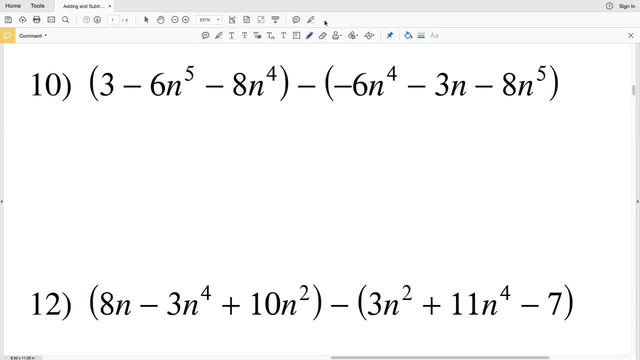 negative 7 K to the fourth, minus 11 K, squared plus 6 is the answer in number 9. lastly, for this video we're going to do number 10. I'm going to start by distributing that negative. so the negative gets distributed to the negative 6 into the fourth, minus 3 n and minus 8 n to the 5th. 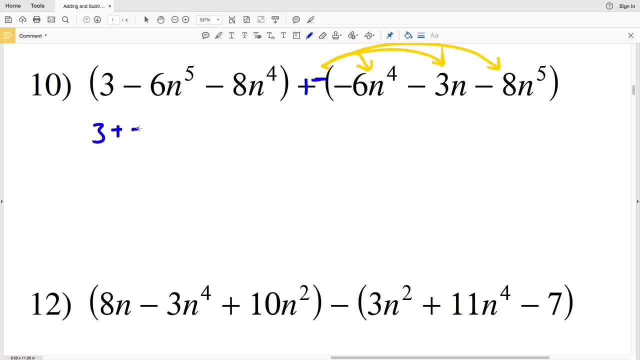 rewriting this. I'll have 3 plus negative 6 into the 5th, plus negative 8 into the 5th. so I'm going to do negative 6 into the 4th plus a positive 6 into the 4th, plus a positive 3 n plus a positive 8. 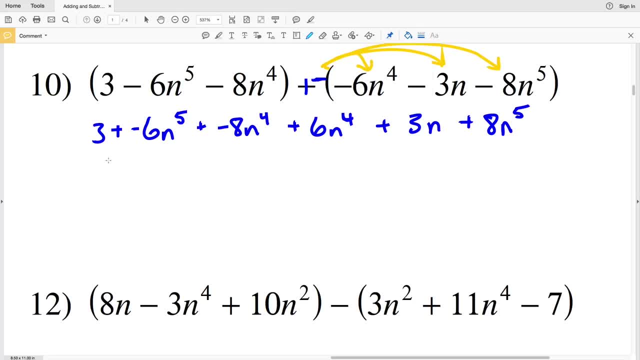 n to the 5th. combining like terms. I only have one constant. I have two terms with n to the 5th, I have two terms with n to the 4th and again I have a single term with n to the first. so combining n. 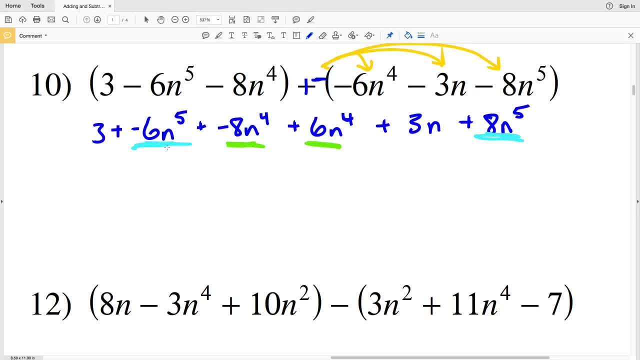 to the 5th to start. since that's the greatest constant, I'm going to do negative 6 into the 5th plus 8 n to the 5th is a positive 2 n to the 5th. now I'm going to combine my n to the 4th I have. 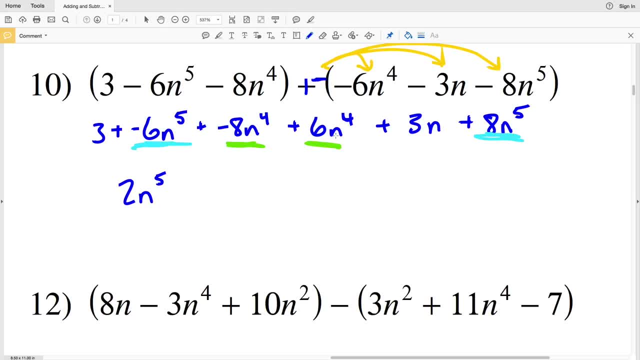 negative 8 n to the 4th plus 6 n to the 4th. we're just going to be a negative 2 n to the 4th, so I'm subtracting 2 n to the 4th. next I will just add the 3 n, since there's no other term to combine. 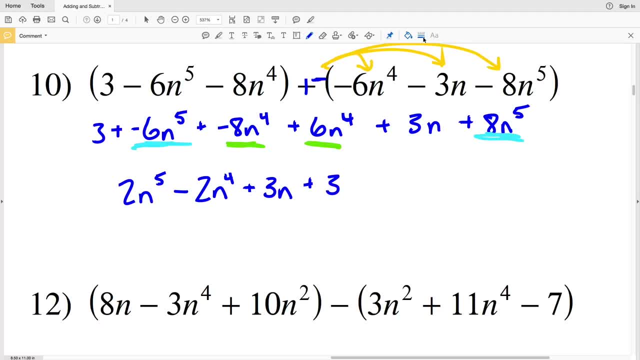 with that and then add the constant of 3, so my 5 n to the 4th is negative 6 n to the 4th. so I'm subtracting 2 n to the 5th minus 2 n to the 4th, plus 3 n plus 3, and remember all likes and 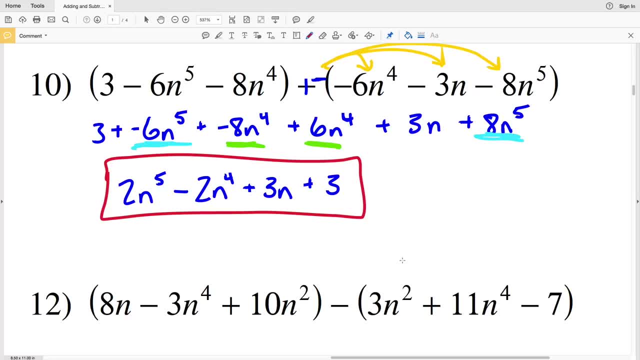 subscriptions are greatly appreciated, so go ahead and feel free to do that now, and if you have any questions, comment below. continue on to the next video, where I'll do numbers 11 through 20. 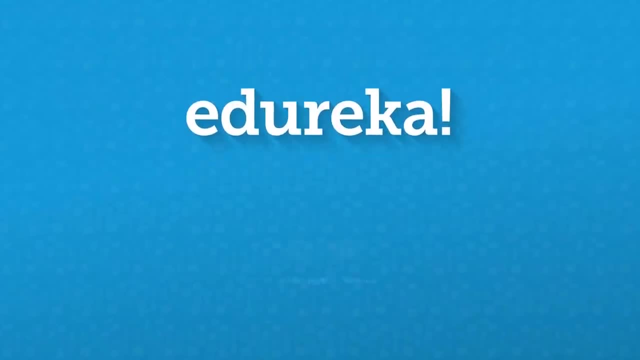 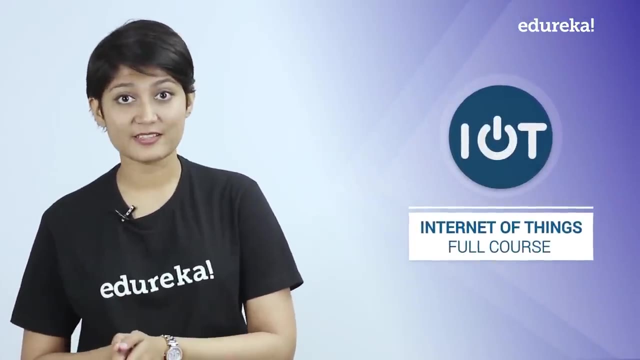 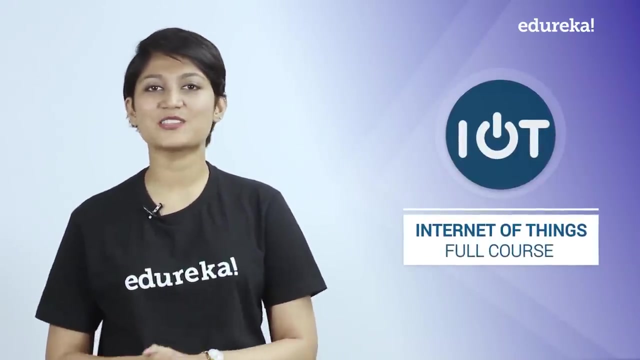 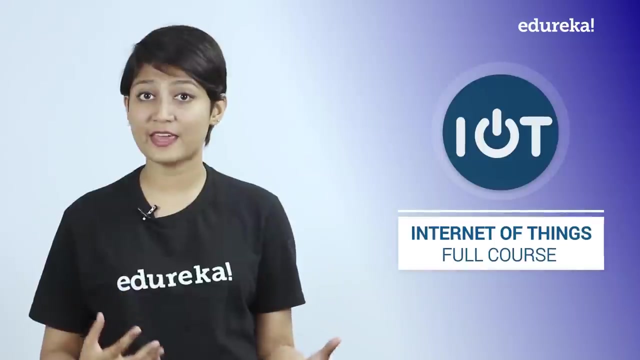 The Internet of Things is a giant network of interconnected devices. These devices are capable of making decisions without any human intervention. Hi all, I welcome you to this full course session on the Internet of Things, and what follows is a series of fundamental concepts on the Internet of Things which will help you get started with IoT. But before, 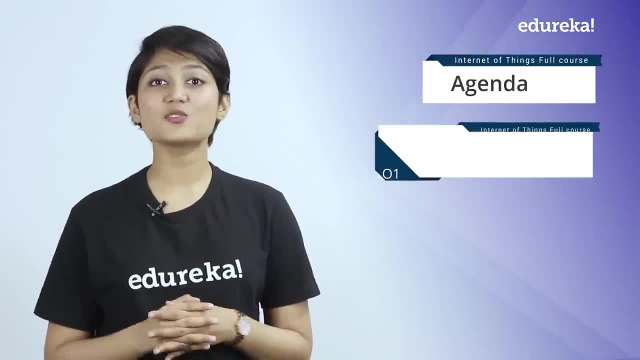 we begin. let's look at our agenda today. So we're going to start out with introducing you to the concept of IoT. We are going to discuss why you need IoT, what is IoT, a few benefits of IoT, followed by a few features and, finally, the very important five-layer. 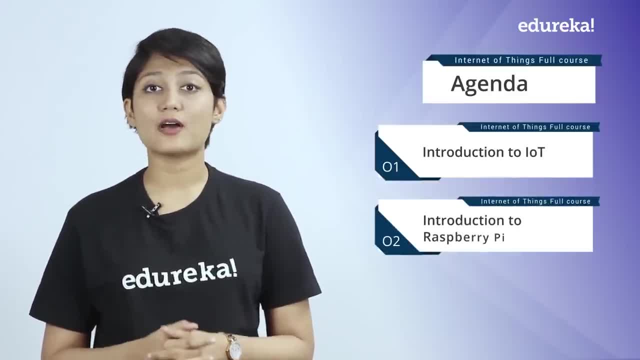 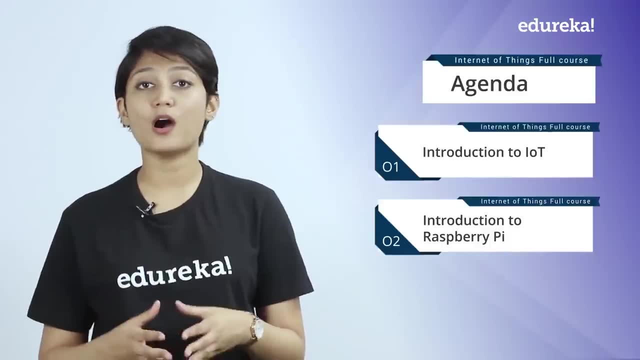 architecture of IoT. Then we're going to discuss Raspberry Pi. In this section, we are going to talk about why you need Raspberry Pi, what is Raspberry Pi, a few hardware specifications and the installation of Raspberry Pi. So let's get started. 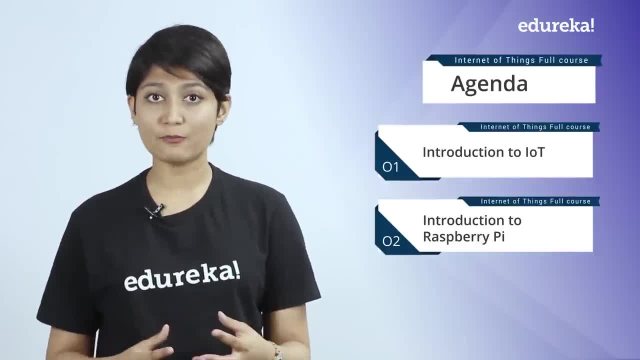 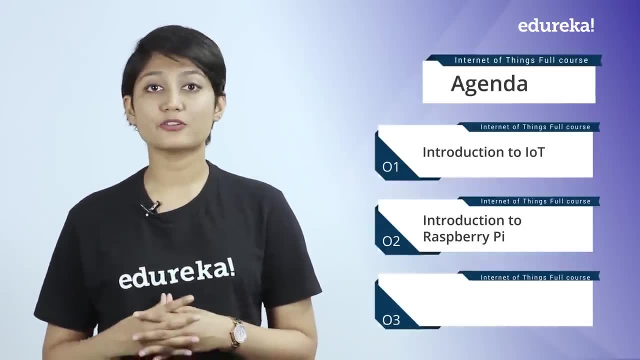 First we will look at the process of creating a Raspberry Pi. Also, in this module we have a few demos, including the Raspberry Pi, a few Sense hats and a Raspberry Pi camera module. Next, we're going to discuss the top seven projects in IoT In this section. 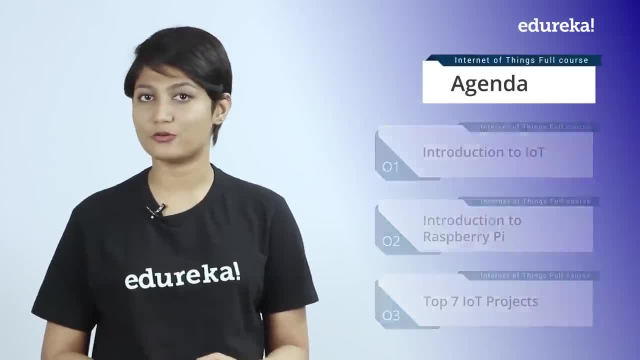 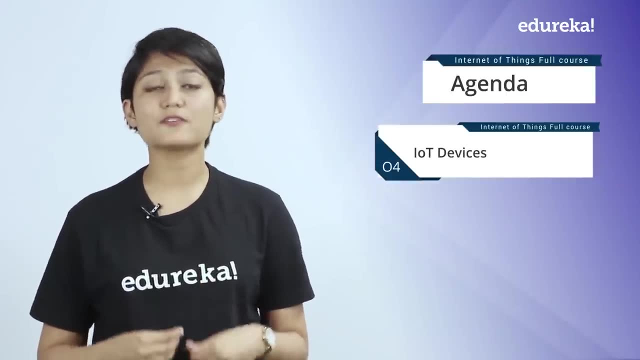 we're going to talk about the best projects that we found in IoT. Next, we're going to talk about IoT devices. we're going to talk about various devices which came into inception after the concept of IoT was introduced. Then we're going to talk about IoT products which